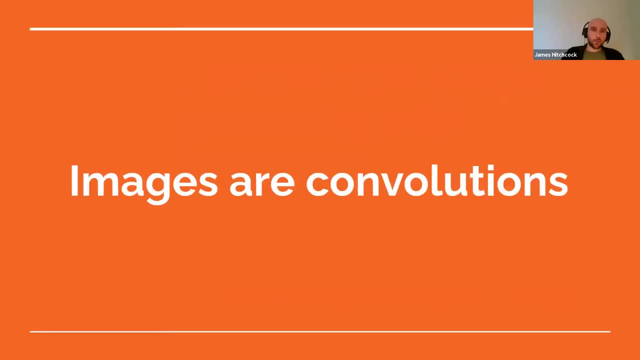 and modeling. So to introduce that, I'll just start with a definition. So this is my practical, working definition of what an image is. So images are just convolutions, specifically two-dimensional convolutions. So telescopes are just analog convolution machines And very many of the useful 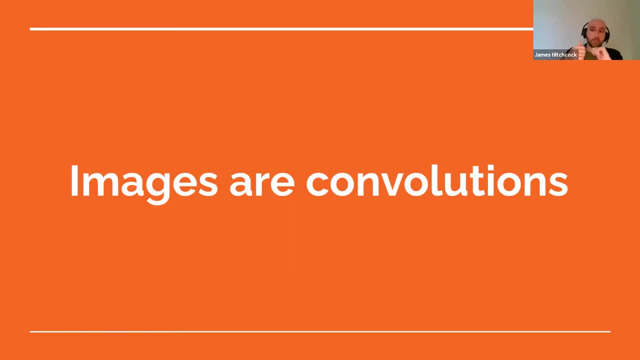 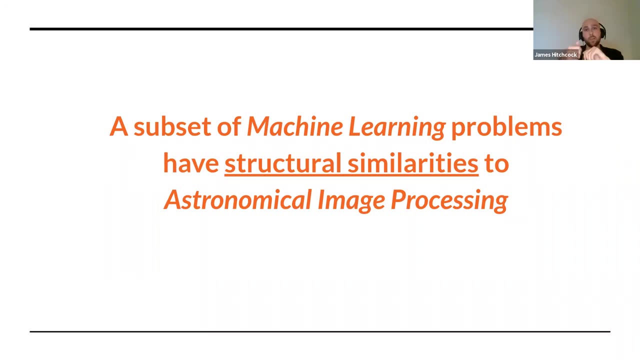 image models which we work with in astronomy can be described as such, And in machine learning world there's a subset of problems that share this structure, So most notably, perhaps, convolutional neural networks. So these are massive models, but they are composed of very many of these two deconvolution operations. 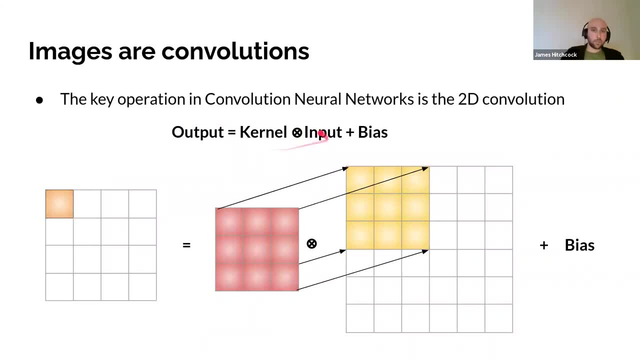 And that operation looks something like this. So we have two images: a small one, which we call the kernel, and a larger one which we could just classify as being the input. And the convolutional neural networks are composed of two components, So we have two models. 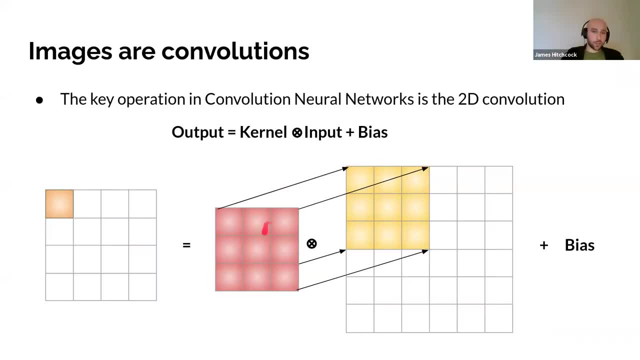 and the convolution of these two things is just the scalar product between the elements in the kernel and the elements in this input, And the kernel slides over the input in some sliding window fashion And then we may have some additive bias term which can be a scalar or another matrix. 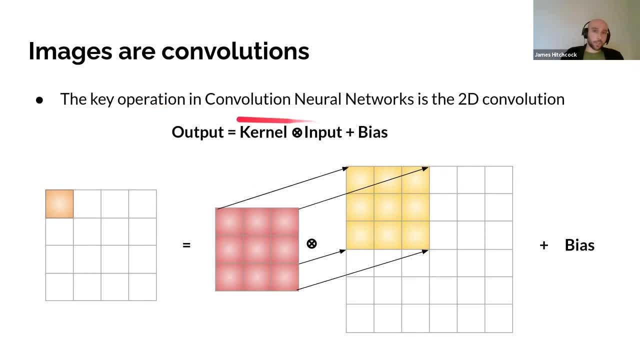 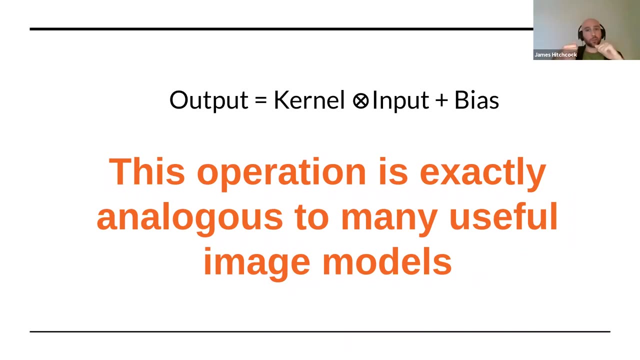 as long as it's the right shape, And then this gives us some output. So this is the core operation in a load of machine learning architectures, And it also happens to be exactly analogous to very many image models that we encounter in astronomy. So just to give you one example, here's the model for an image as observed by a telescope. 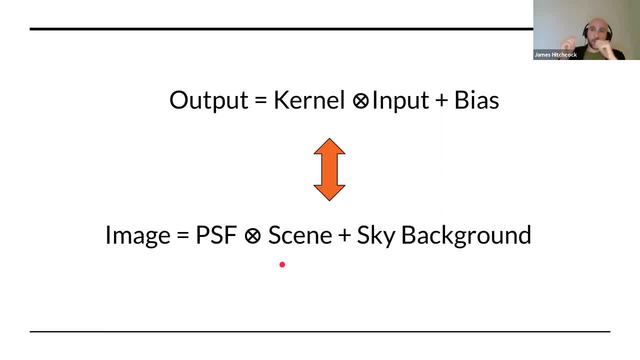 And so if we point our camera at some astronomical scene, that thing then gets convolved with the points for function of the observing system, And then we have something added onto the end, some smooth background. So there is this quite striking similarity, which is that this is a very interesting structure, And so the idea behind what I've been working on is: 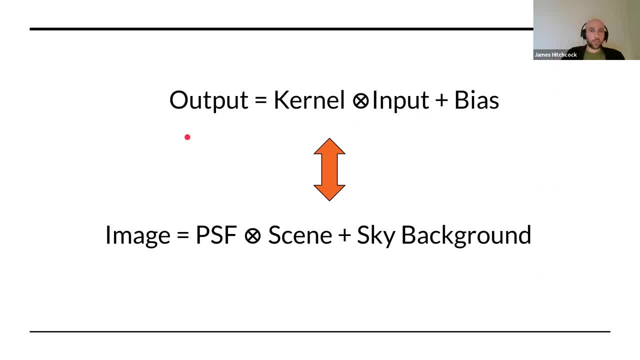 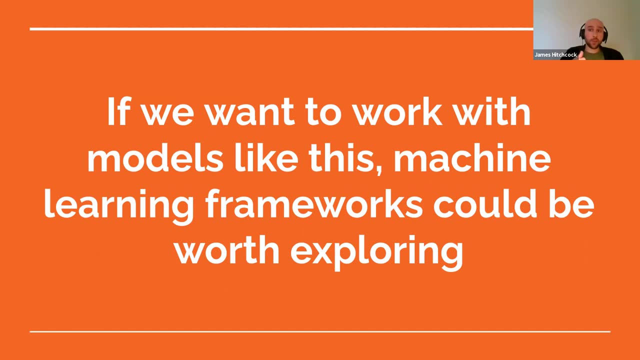 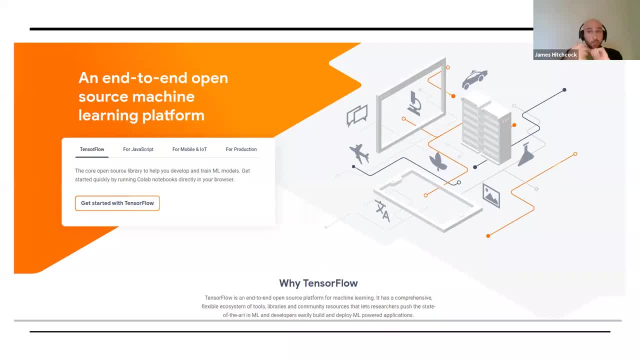 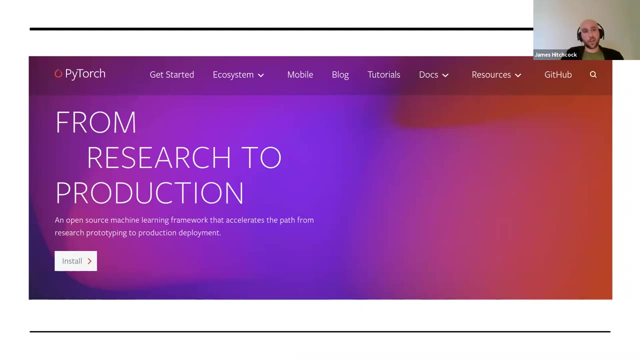 And machine learning frameworks, The first of which was pie torch- Sorry добlo- Which was released in 2015.. And the following year, PieTorch came out, And by the title of the talk you'll probably guess that I ultimately went with pie torch. 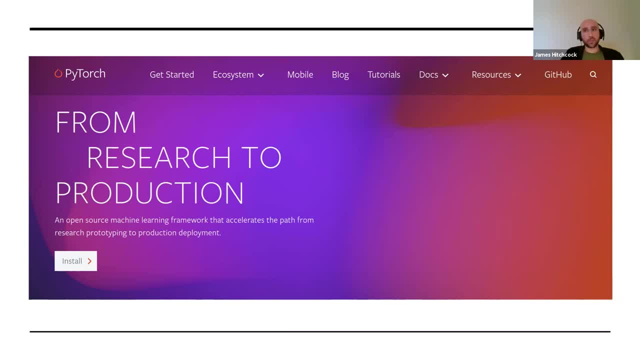 The simple reason being that I just prefer the syntax and the documentation. Like most astronomers, I pretty much coosably work In Python these days. curve to getting to grips with this stuff was pretty shallow, But everything I'm describing today that I've applied in PyTorch as far as my wear can be achieved in TensorFlow and similarly. 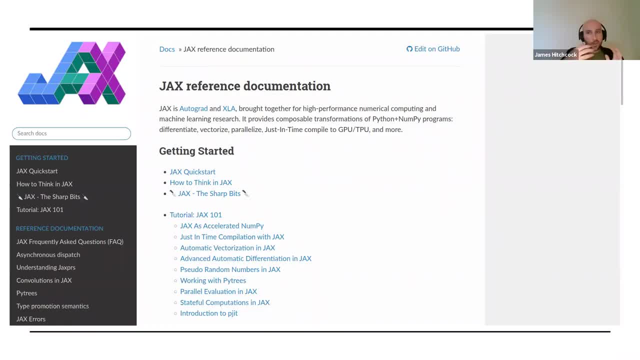 could be achieved in Jack, So this is the new kid on the block. This was released by Google in 2020 and if you're unfamiliar with either PyTorch or TensorFlow, this I would suggest be the first port of call. if anything I say today sounds interesting and worthwhile trying in your own. 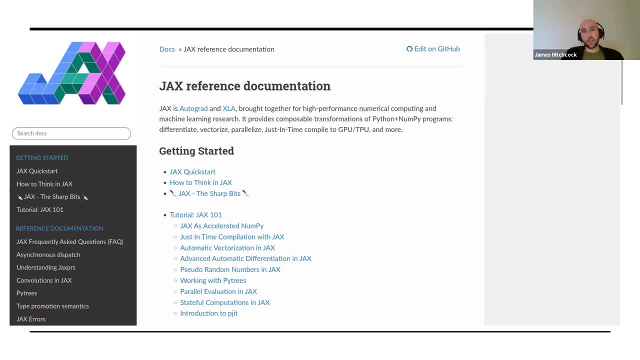 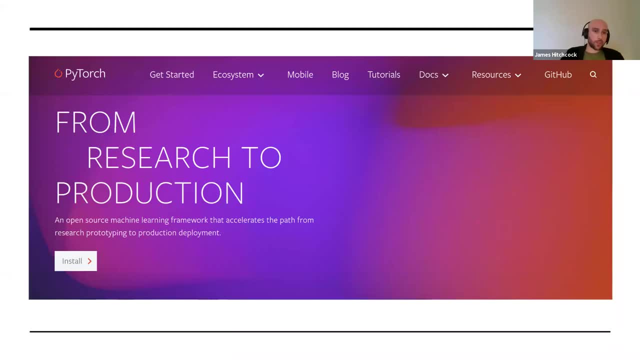 research, simply because if you have any NumPy code, this thing can be used as a drop-in replacement for that. But just going back to PyTorch, so you'll see that this thing is described as this open source machine learning framework. That's a good definition of how it's normally used. but for 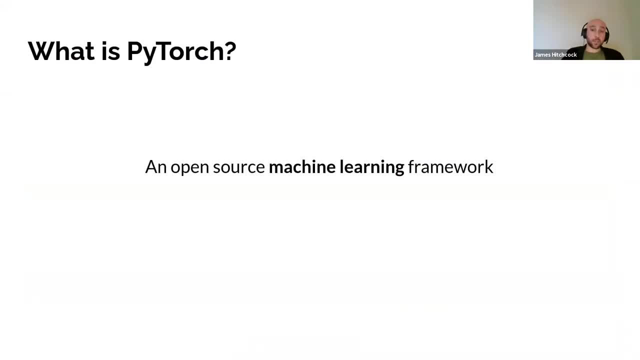 the purposes of my own research it's a much more useful definition is to drop the machine learning element altogether And just think of this as some generic modeling tool. So just to be absolutely clear, because I understand the title of this talk can be somewhat misleading. I don't do machine learning, but I am. 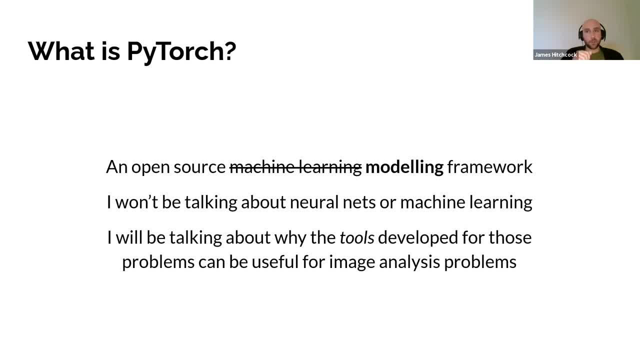 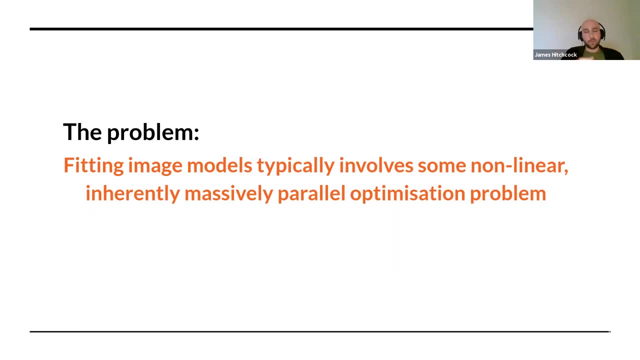 trying to repurpose the tools for some specific image modeling problems that we encounter in astronomy. So I guess the next step is to just specify what that problem is. So I fit image models to data And this will typically involve some non-linear but inherently massively parallel optimization. 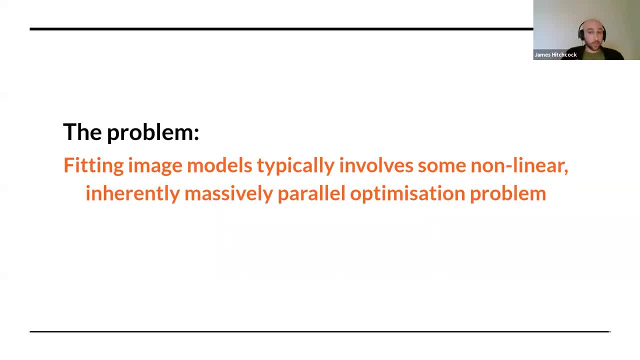 problem. So these optimizations are non-linear because we have to contend with photon noise, So this is Poissonian. So the variance is dependent on the models. It's dependent on the expected number of counts due to photon counting statistics But operations on images. 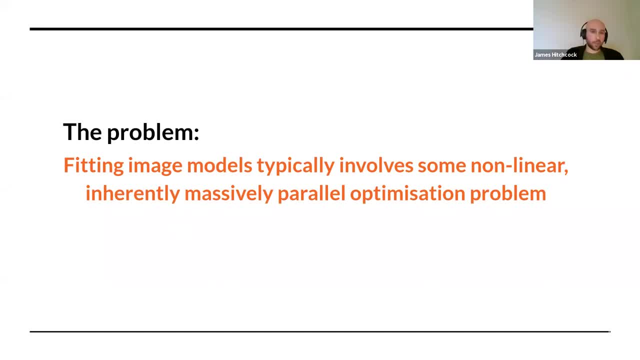 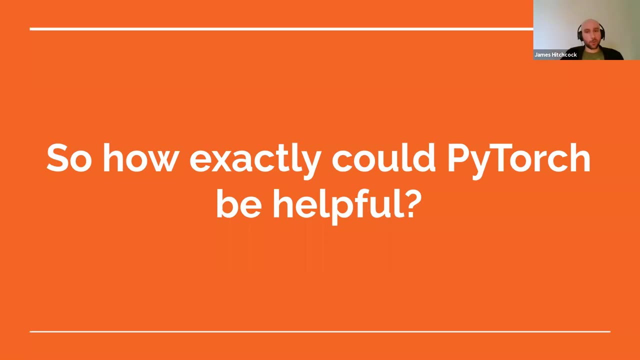 are embarrassingly parallel in the jargon, because operations that we perform on pixels are independent of all other pixels in the image. So if you have the right hardware you can potentially exploit that. So how on earth is PyTorch useful for addressing that sort of problem? So getting 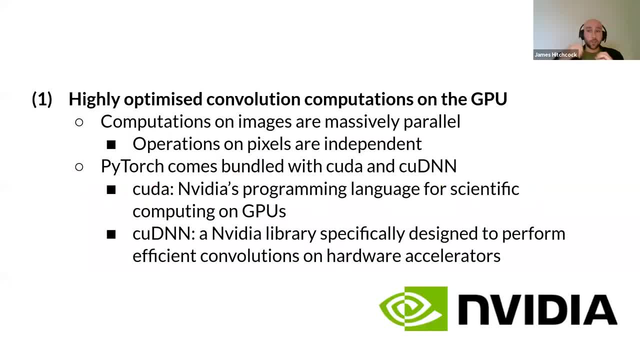 into specifics now. So, first off, these frameworks come with highly optimized convolution computations that you can easily run on the GPU, And I stress the word easily there. So PyTorch, it is a PyPonic tool, but the functions that you're calling are going to be either written. 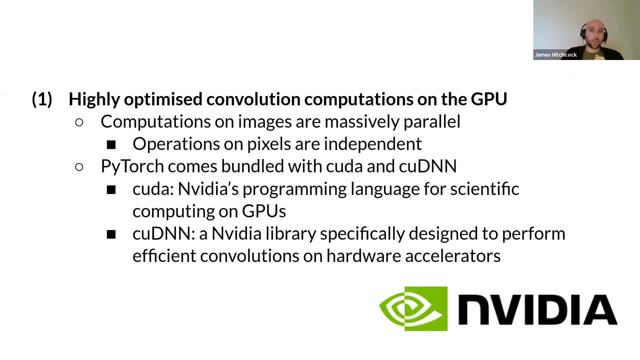 in C++ or in CUDA, So it's performant while still being nice and readable, and development is usually pretty quick. So CUDA is NVIDIA's GPU-specific programming language, And PyTorch comes bundled with this and other nice accessories like cuDNN, right out of the 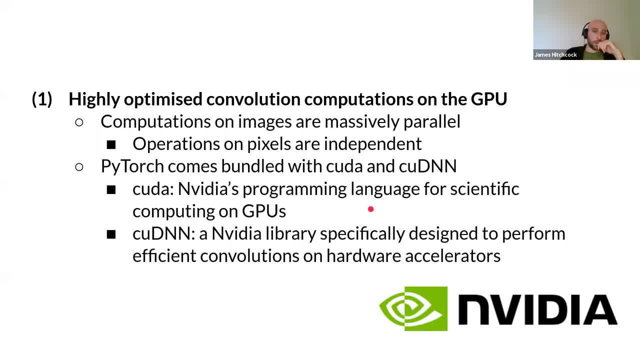 box. So in the context of convolutions in particular, this cuDNN tool is particularly useful because this automatically, that is, behind the scenes, takes care of the previously somewhat challenging task of memory management, like moving in some optimal way a memory onto your 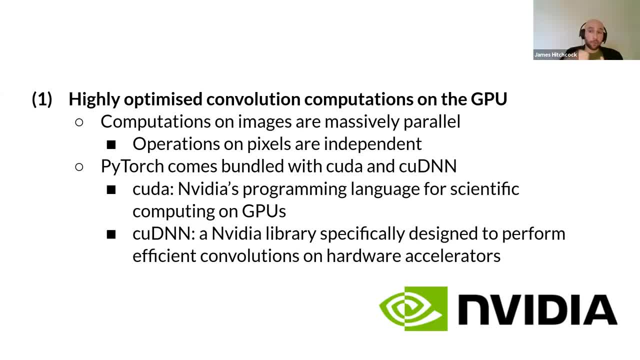 computers. And also it comes bundled with efficient algorithms for performing convolutions themselves. And again, that's all taken care of automatically for you, So you can just focus on the science and the program aspect, like the technical details of the GPU, programming is. 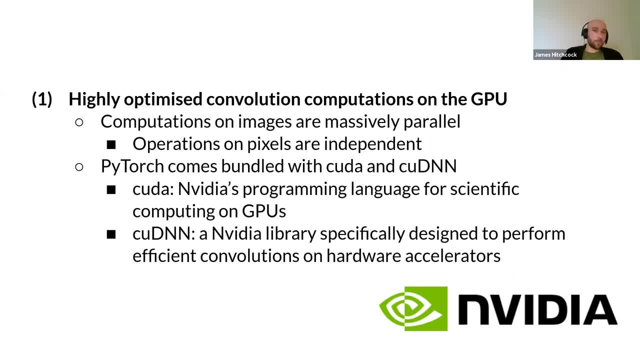 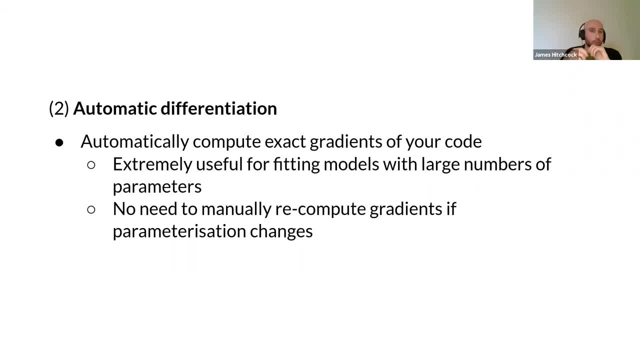 done automatically, So that's very useful. The second feature is automatic differentiation. So image models. Now, I'm typically fitting models with a least the order of a hundred parameters, if not thousands or tens of thousands. So if you're fitting large models like this, it's incredibly useful to have exact gradient information. 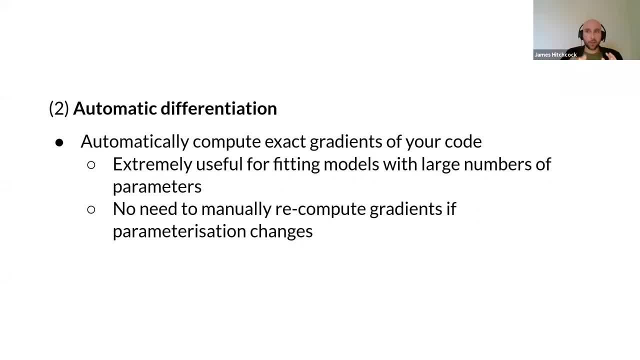 Numerical, noisy approaches to optimization just will typically fail in that larger parameter space. So that's very useful for that reason. And a secondary benefit of this tool is that you have a certain flexibility here with reparameterizing models and trying out different models. and 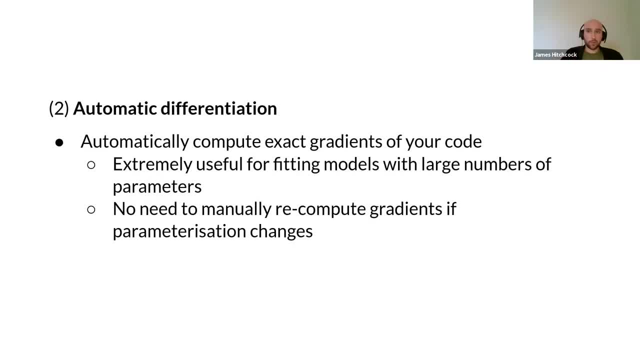 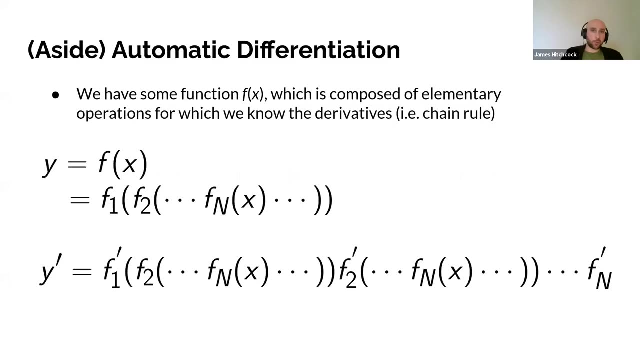 different problems, Because if you're trying out different models and different problems, because of the fact gradients are computed automatically, you don't need to manually recompute these every time you change the parametrization, So that makes experimentation quite straightforward. It's an equality of life feature. So just briefly if you're unfamiliar. 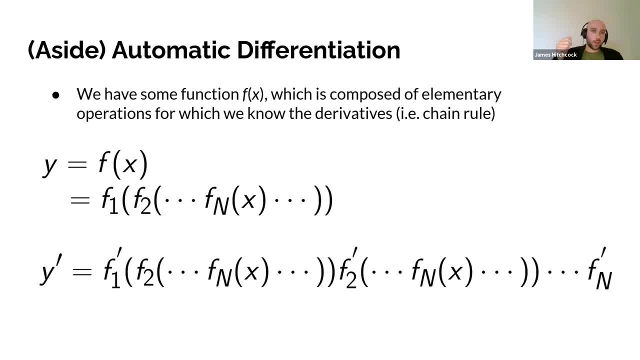 with how this works, just to give a very high level overview. automatic differentiation is basically the chain rule applied to code. So say, we write some function in code, some function in the code, and then we compute the derivative of x, which might be your objective. 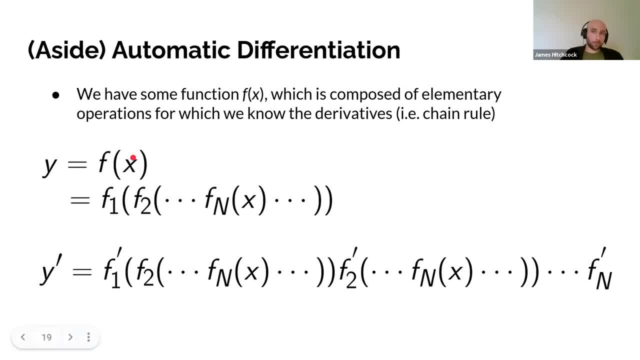 function in an optimization scheme. Although we don't know the derivatives of this thing with respect to our model parameters that we're attempting to fit immediately, we can recognize that we can decompose pretty much any function into a sequence of simple elementary operations. So additions, modifications, exponential functions, trigonometric functions, And we can compute the. 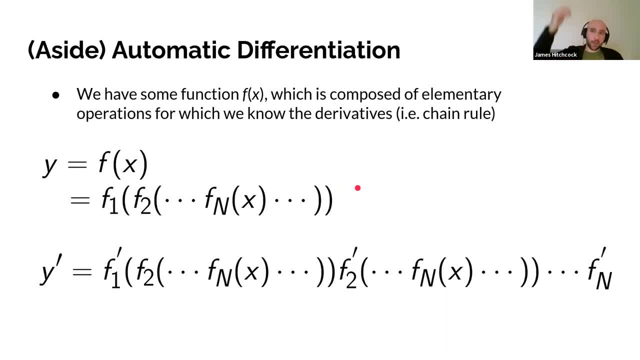 derivatives of those. So those are simple derivatives to compute. So if we make a graph of all that sequence of operations, we can just then work backwards through it, just applying derivatives as we go, just by applying the chain rule, and then ultimately end up with the derivatives with respect to our input parameters. 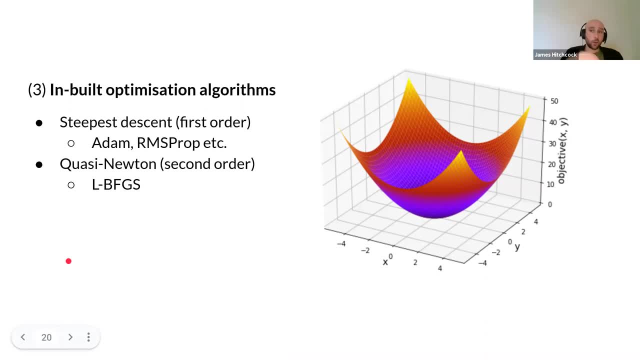 The third tool- and this again is more of a quality of life feature- the optimization algorithms are built into PyTorch And there's a nice flavor of both first gradient methods and first derivative and second derivative approaches. And what's quite good about the way that PyTorch 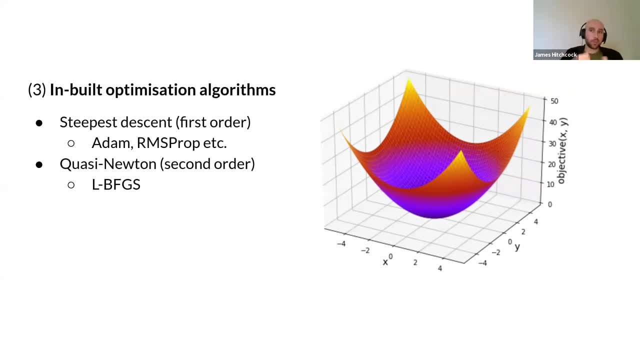 goes about its construction of computational graphs and auto diff means that you can switch between these approaches, which sounds kind of odd, but for complex optimization problems that can be useful, Because if you're working on time, critical science cases and you need to fit models quickly, it can be beneficial to start. 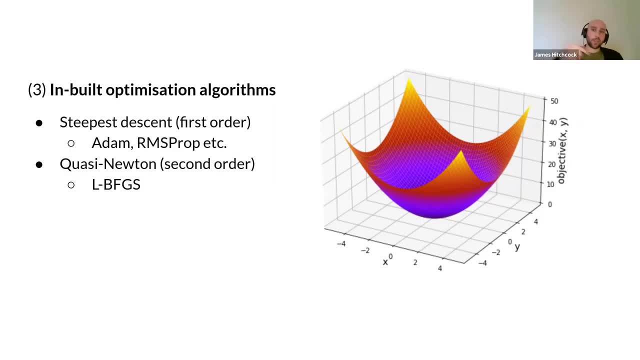 with just simple, inexpensive first order methods that get you at least in the ballpark of where the minimum is and then just switch to some more sophisticated second order methods once you're there and hopefully then you can converge quite quickly. So if we put those three ingredients 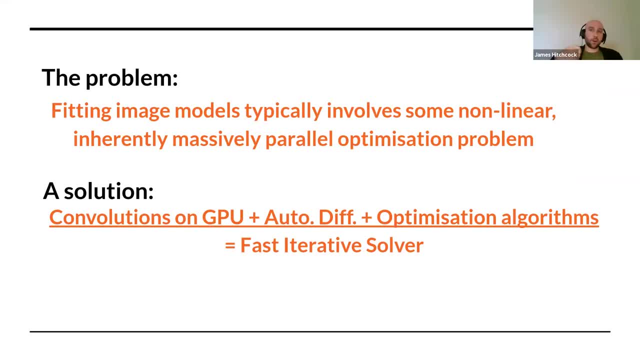 together we've effectively created some fast numerical iterative solver, which happens to be exactly the sort of tool that might be useful for addressing image modeling problems of this form. So we can compute the forward model in an optimization scheme very quickly because we can do fast convolutions on the GPU, And then we have exact gradient information and 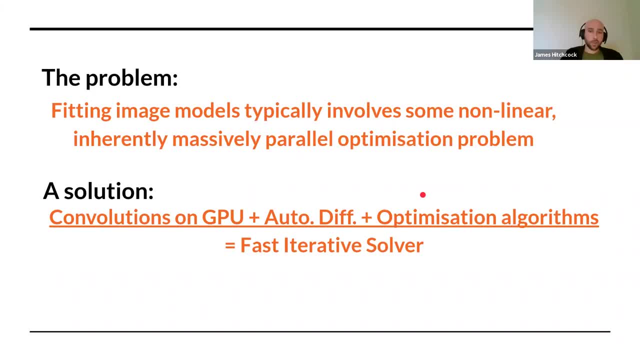 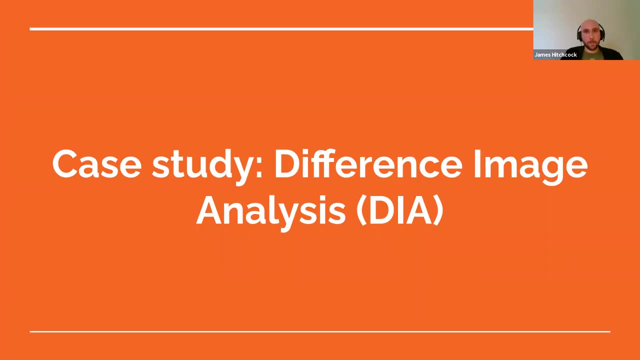 some nice optimization algorithms to help us converge. So moving on to so I mean, this all sounds kind of nice in theory, so I'll now outline an actual application of this, So namely a difference image analysis or image subtraction, which I'm sure many people in this community are familiar with. 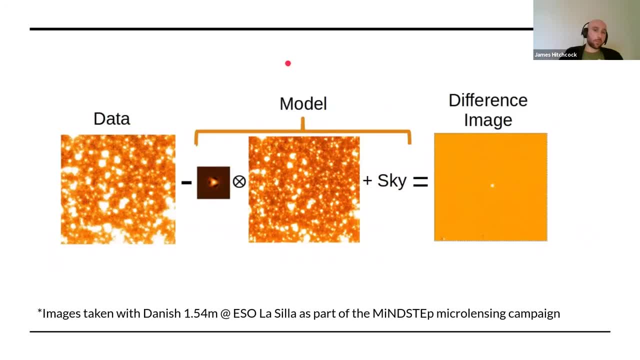 But just to give a brief overview. the basic idea is, if we have two images of some astronomical scene taken at different times, we want to fit some model that corrects for the systematic changes in observing conditions between the times these two images were taken. And we can do that by 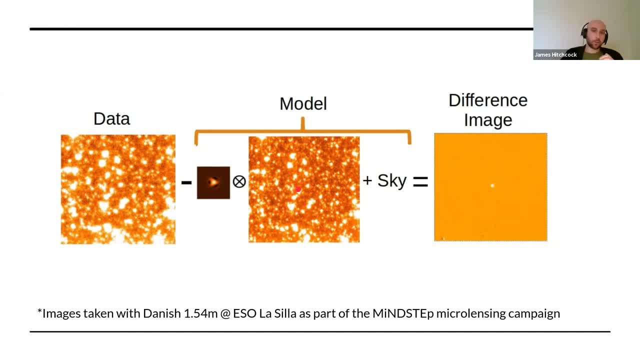 choosing one of- well, either correct or incorrect, constructing or selecting some high quality, high signal to noise, high resolution reference image or template image and then fit for this object what we call the convolution kernel, which corrects for systematic differences in the shape of the PSF And also it encodes differences. 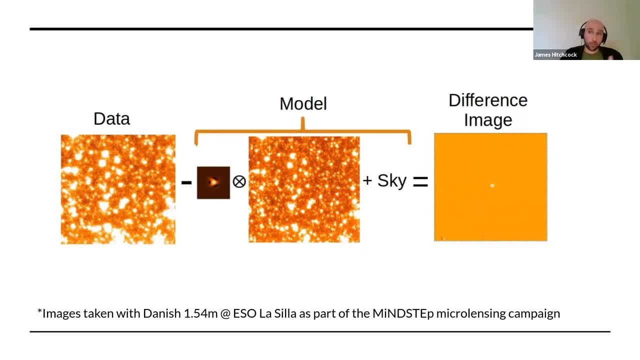 in atmospheric transparency and exposure times, so your photometric throughput, And then we can also fit for changes in the sky background too. And once we have that model, we can then subtract it from our data And this gives us an image of a different image which shows up any variability between the times these two images have been. 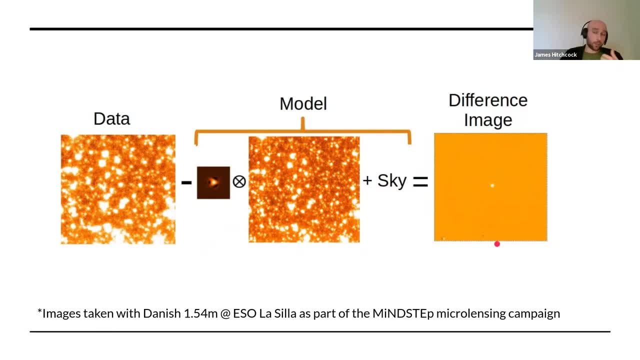 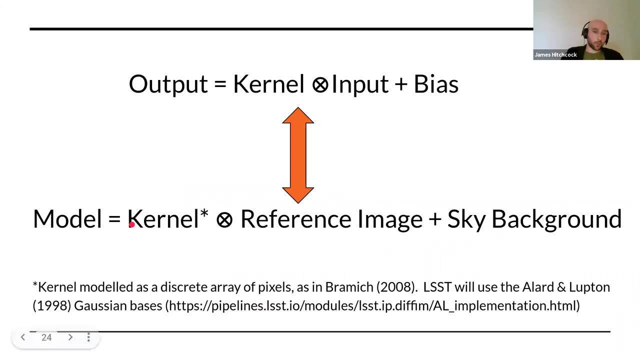 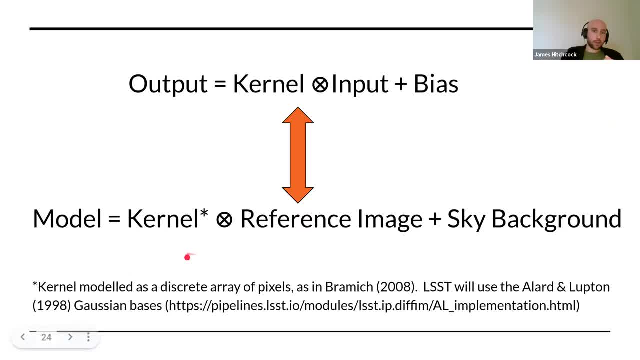 this structure that I introduced And, I suppose, just a technical detail here. You do, of course, have a choice of how you want to model the kernel. Throughout this talk, I'm assuming it's modeled as a discrete array of pixels. LSST will do something different in their image subtraction pipeline. 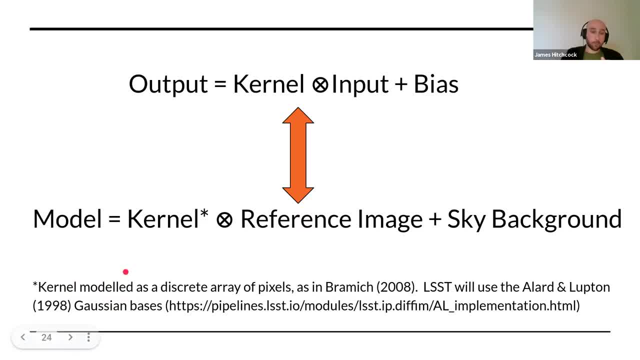 and they adopt a Gaussian basis for how they, how they model the kernel, The, the, the discrete array of pixels, is effectively just a delta function basis. So it is somewhat more flexible than the Gaussian basis, but it is more computationally expensive. 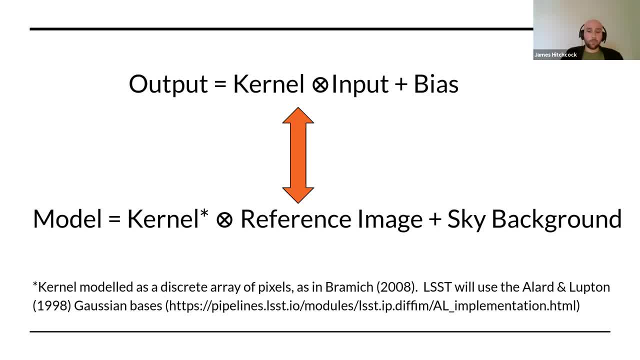 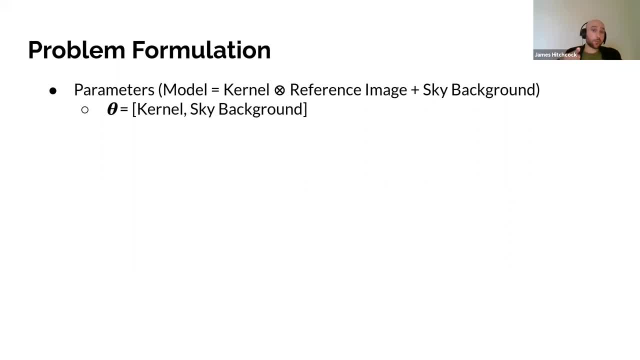 to work with because you're fitting in more parameters. So there's just something to be aware of. So okay, So we, we we specified the forward model, a parameterized forward model. We want to fit for this kernel and sky background term. So the next step is to write down a noise model. 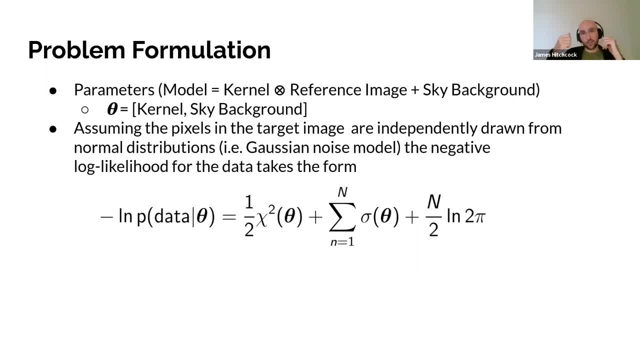 and a convenient way to do that is with the likelihood function. So for conventional astronomical imaging where we have observations that in exposure times of tens of seconds and we're observing with CCDs we can reasonably adopt a Gaussian noise model And the equipment and the negative log likelihood of that looks, 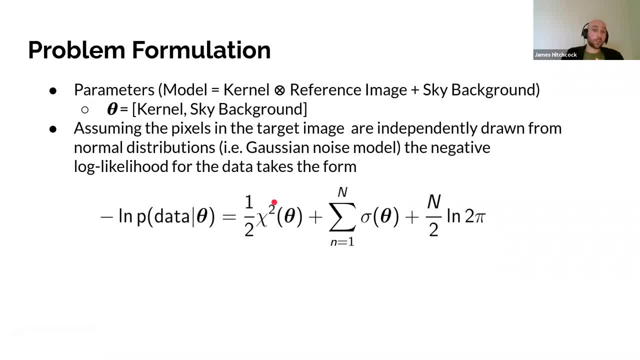 something like this. So just to walk through the terms here. So this is just the familiar chi squared, So the square difference between the model and the data over the variances. This is, of course, a function of model parameters, The the thing to note, though. 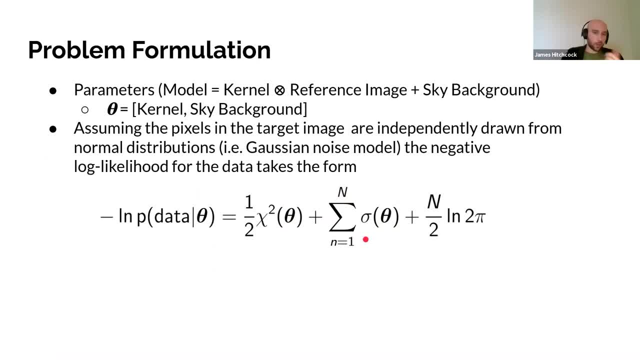 is that we also have this additional term here. So we have chi squared plus these, these things here which are our uncertainties on the pixels in our image, And these two are functional model parameters because of photon shot noise. So this is where the non-linearity enters. 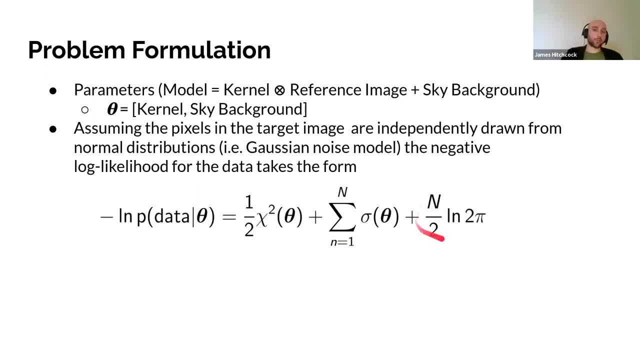 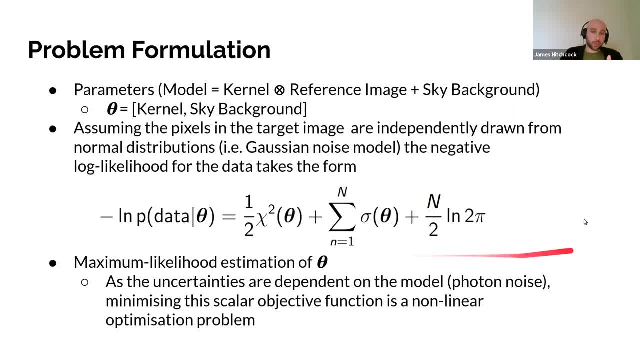 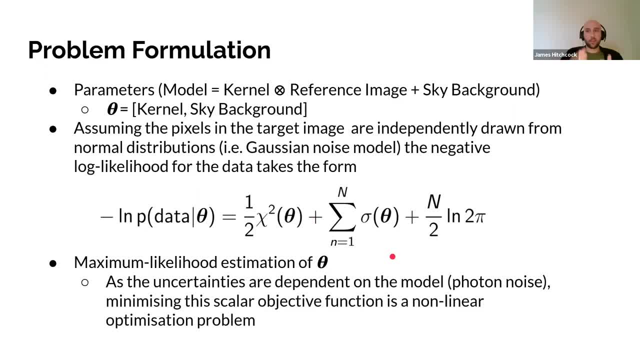 But because of the non-linearity here we can't do that analytically, so we need some numerical solver, which again is exactly the sort of thing that we've just built from the those workpoints one, two, three within Pytorch. So you know, we need to compute the forward model at each. 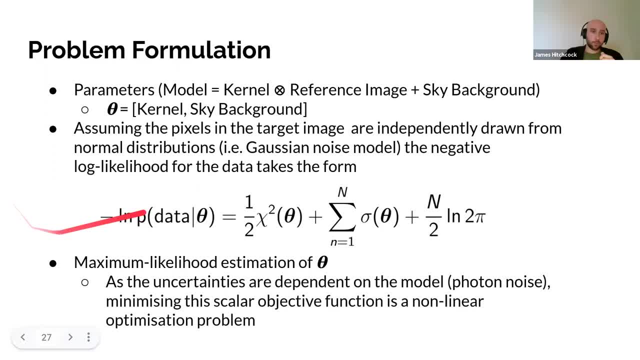 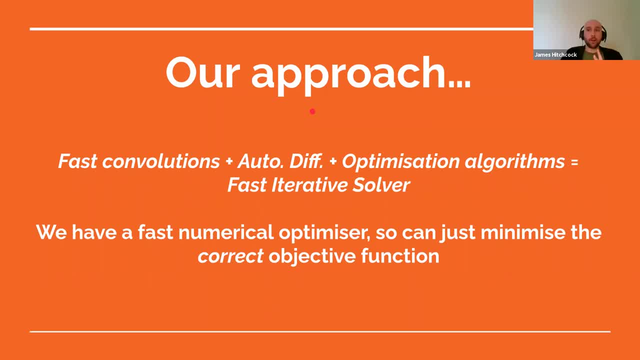 iteration and update our parameters with respect to this or this loss function is negative block likely function. So before I show you some results of this, I'd just like to contrast this with the classical approach of solving this problem, Because, you know, we, in our framework, because of GPU, because of running the convolution computations in GPU, we can do this whole thing very quickly. 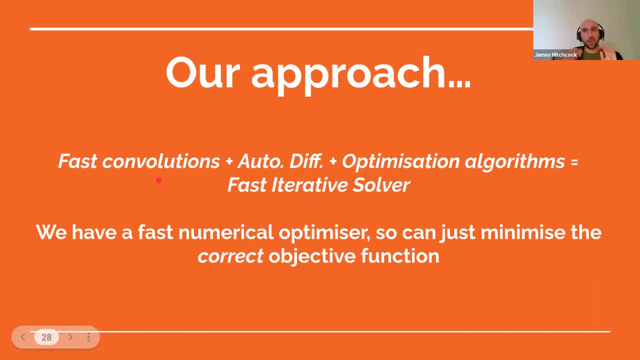 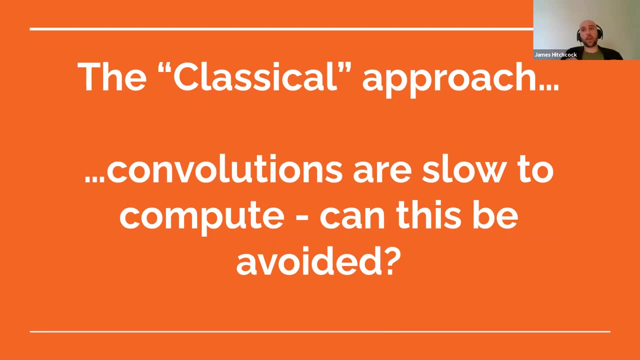 Of course, if you're attempting this on the CPU, it would be incredibly slow, And this is the problem classical approaches had to contend with. So the idea is: well, can we reformulate this problem and bypass direct convolution computations altogether? So this is kind of similar to how LSST is approaching this problem. 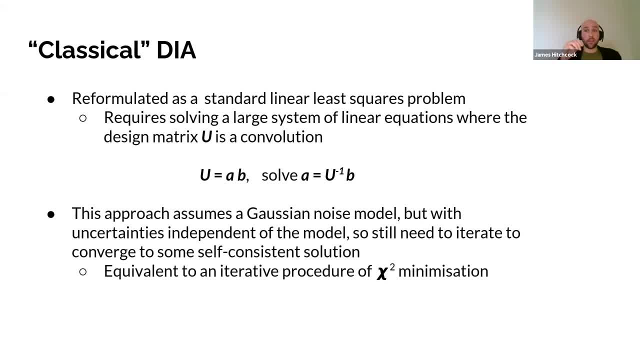 And you can by reformulating it as a standard linear least squares problem. So again, you're assuming a Gaussian noise model here, But you're dropping this. You're assuming the dependence of your uncertainties on your model parameters, But this does allow you to then reformulate it as a standard linear least squares problem where we can specify a design matrix to represent the convolution. 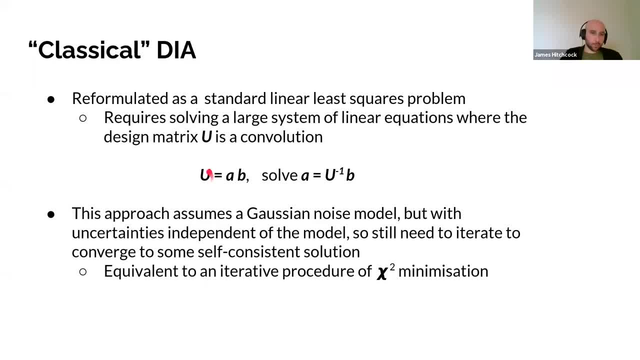 So we're not doing direct convolution computations, but we can represent it as this matrix, And then we just need to set up some data vector And then, using the power of linear algebra, we can efficiently solve this system of equations. Of course, the issue here is that you've made a problem that is in reality nonlinear a linear one. 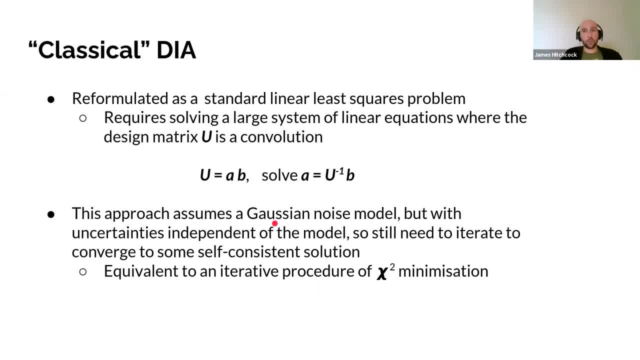 So, in order to converge to some self-consistent solution, you still do need to iterate. So the way that will work is: when you first construct these matrices and vectors, you need to plug in some initial estimate for your uncertainties. Then you can solve the system of linear equations. 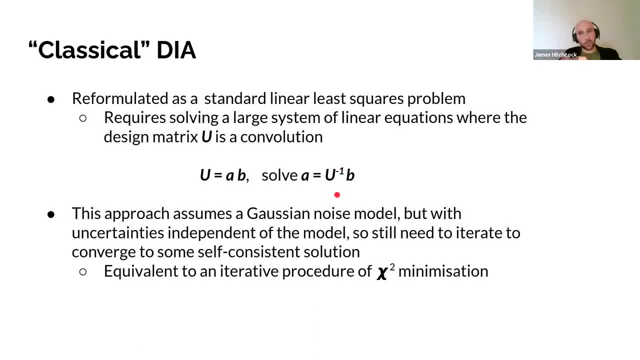 You get some estimate for your model. You can then update your uncertainty estimates And then from scratch again reconstruct the system of linear equations, solve it again, update your uncertainty estimates and proceed in that way. So this is basically just an iterative process of chi-square minimization. 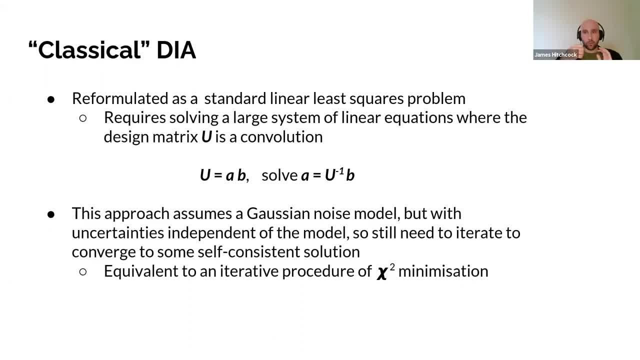 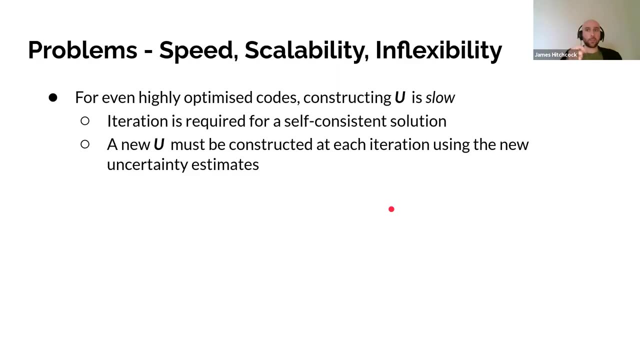 And then, hopefully, within three or four iterations of doing that, you'll converge to some consistent solution, And this works pretty well. But there are of course some problems here, Namely speed. So although you're bypassing direct convolution computations, you still need to specify the convolution as a matrix. 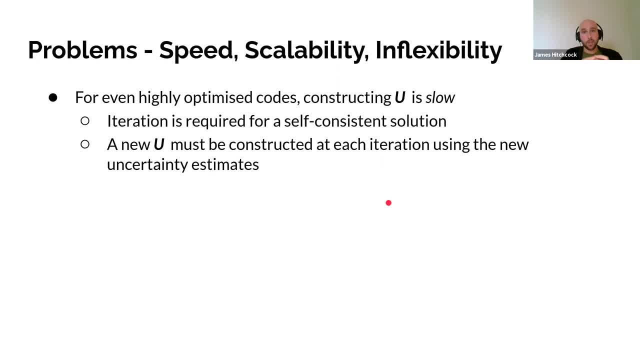 And just constructing that matrix takes a long time. Again, this is more of a problem for the delta function basis representation of the kernel, because there are many parameters And you need to write basically just a lot of nested loops to build this thing. So this is the bottleneck of this whole process. 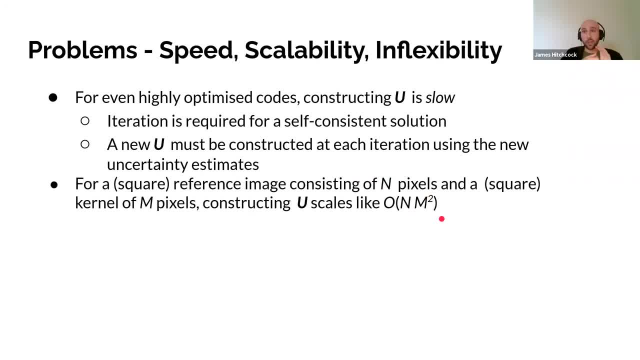 Also the scaling with the number of parameters in that kernel. So this is the bottleneck of this whole process. Also, the scaling with the number of parameters in that kernel is somewhat unattractive in that it goes with the number of parameters to the power of two. 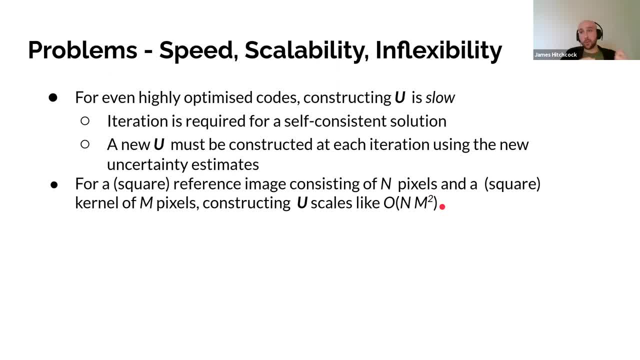 Again, this is somewhat naive scaling. I mean, there are ways to exploit the symmetry in the construction of the design matrix, But as you'll see later on, I'll use a naive scaling for our method two. And then a third point. quite an important point is the inflexibility of this classical 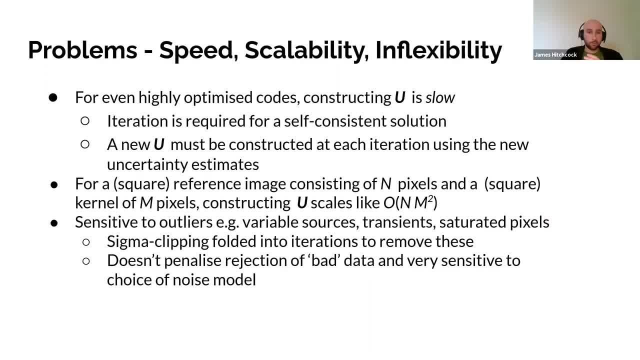 And then a third point. quite an important point is the inflexibility of this classical approach. So you are explicitly assuming a Gaussian distribution for the noise. Gaussian distribution is very tight, So they're very sensitive to outliers. If you're doing a regression under Gaussian noise models in the presence of outliers, the fits can be badly affected by those few points. 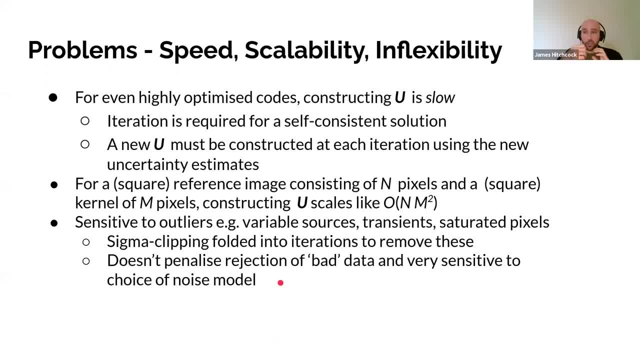 So, in order to make sure our answer isn't sensitive to them, a sigma clipping procedure must be folded into that iterative process. So, in order to make sure our answer isn't sensitive to them, a sigma clipping procedure must be folded into that iterative process. 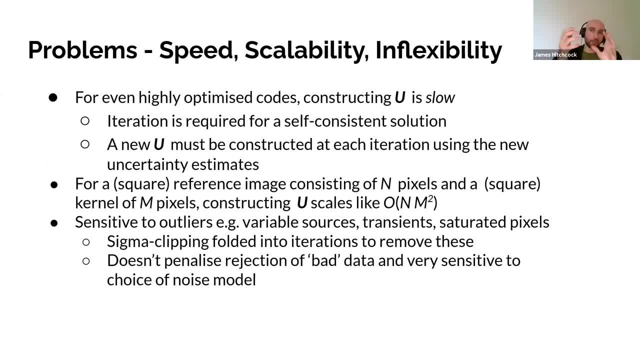 So, in order to make sure our answer isn't sensitive to them, a sigma clipping procedure must be folded into that iterative process, So lashing out of thinking about a likelihood answer or the process of reconstructing the matrices, solving the system and then updating uncertainty estimates. 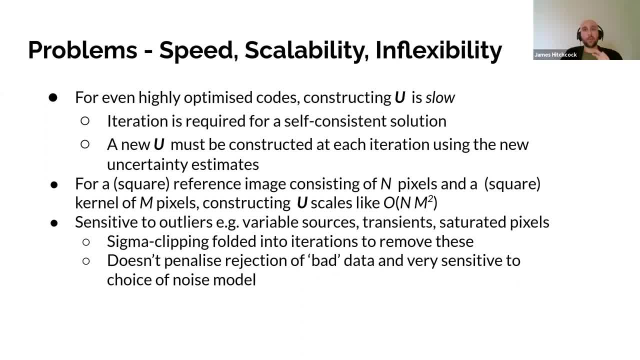 Of course, there are general issues with sigma clipping, about throwing away data, But this also, of course, complicates this issue of convergence, because you're throwing data away at each stage, So it does again, in combination with this slow construction of design matrix, cause some issues. 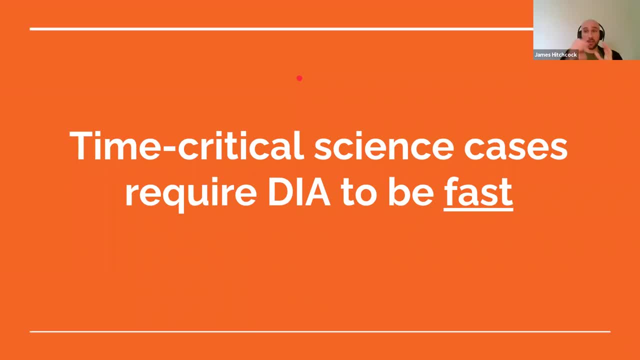 But yeah, I want to highlight because, particularly for this community that deals with time, critical science cases we require: the faster we can subtract images, you know, the faster we can issue alert streams and the more science we can do, because the faster we can detect transient astrophysical 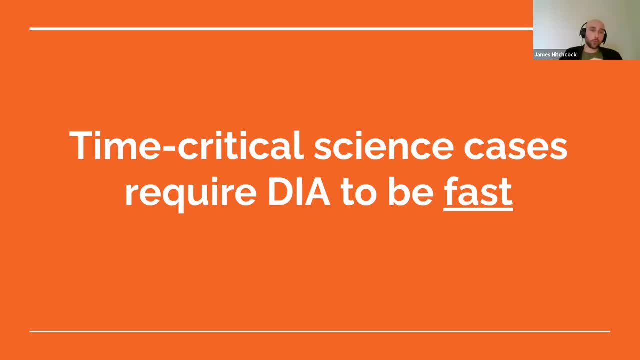 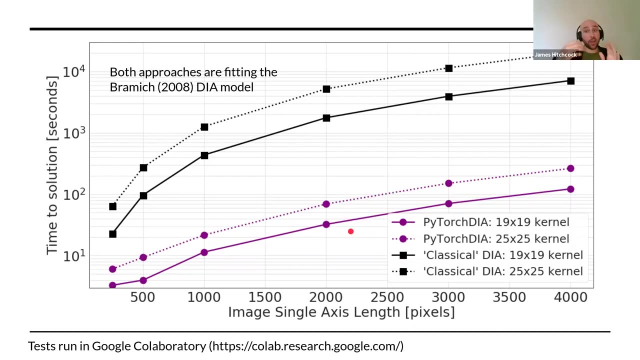 events. So I'll just show you some performance comparison tests here. so in purple here, this is PyTorch DIA, so this is the software implementation of the, this fast numerical iterative solver that's been implemented using PyTorch, and this is all run on the GPU and then we have its classical 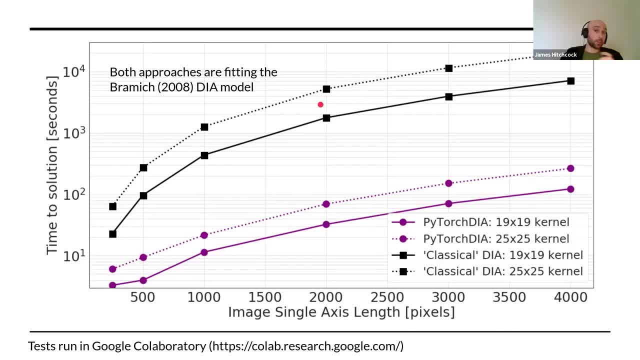 analog here in black, and this is: this is solved on the CPU and all computations have been done in Google Collaboratory, so the hardware is equally modest or at least modestly comparable. so hopefully isn't too and unfair Test here, because of course we're using different hardware to solve this problem. 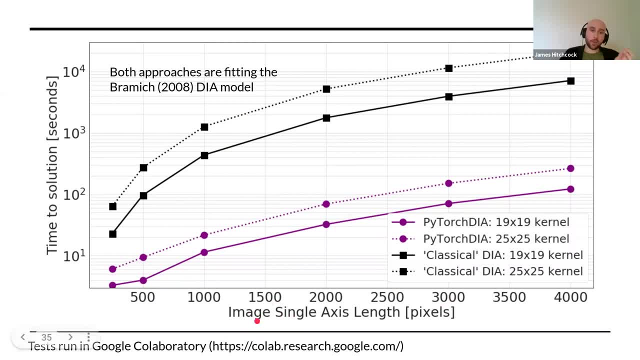 and just on the x-axis here, this is the single axis length of the image. so, and these are square images, so an image of length, 1000, one axis, has a total of a million pixels in it and these are just the solution. times, the time to fit our DIA model and you can see, you know, for 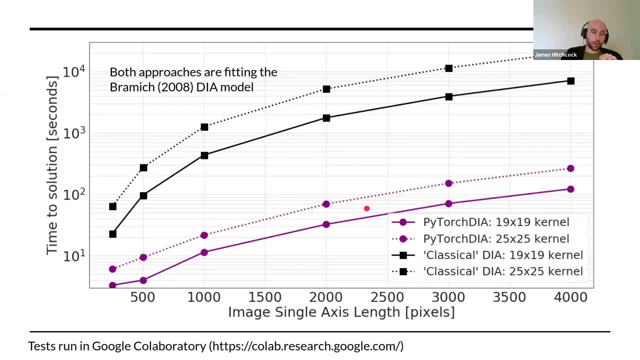 different image sizes and kernel sizes. the PyTorch DIA is at least an order of magnitude faster than the classical approach to solving this problem, and also so the difference between the dotted and straight lines here, or undotted lines, are an indication of the scaling with kernel size and the relative difference between these. 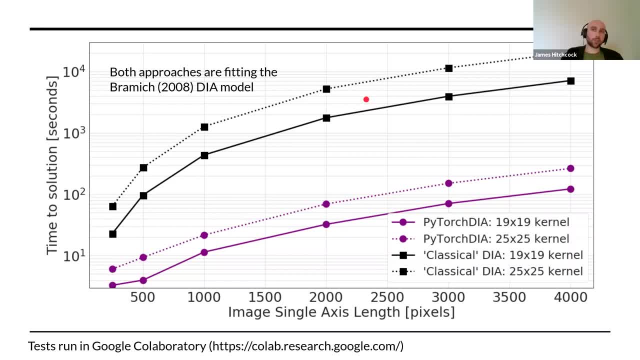 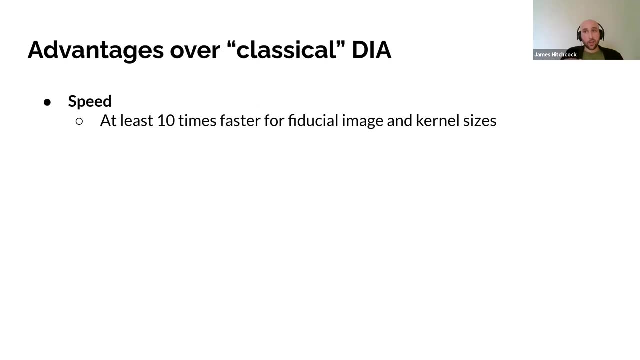 two lines is somewhat smaller than the classical approach, so it suggests that our scaling with as we increase the number of parameters on our model is also somewhat better. So just to summarize, so some of the advantages of this approach over the classical approach are the speed, the scaling and, as I briefly mentioned, these are naive scalings for both approaches because 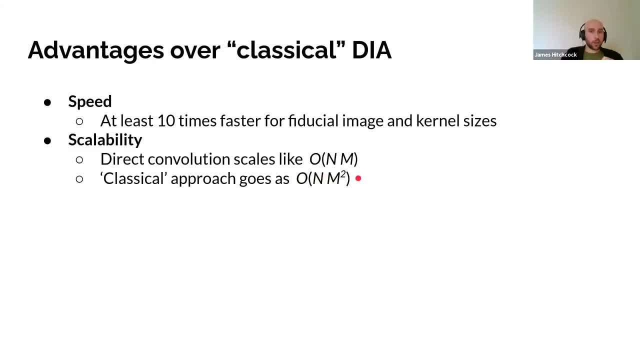 in the construction of the design matrix. for the classical approach you can again exploit symmetries in the problem to speed this up a bit. but because of the special NVIDIA libraries that PyTorch uses under the hood, the scaling with kernel size isn't necessarily linear as it would be for a 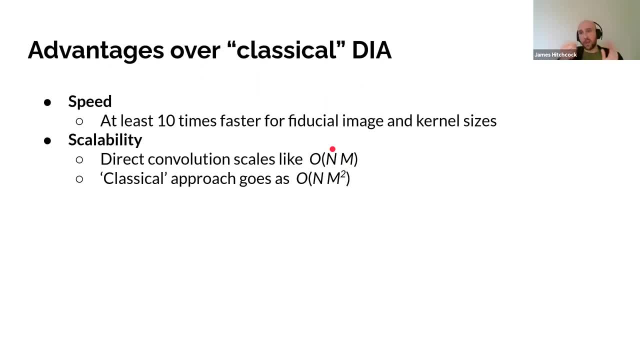 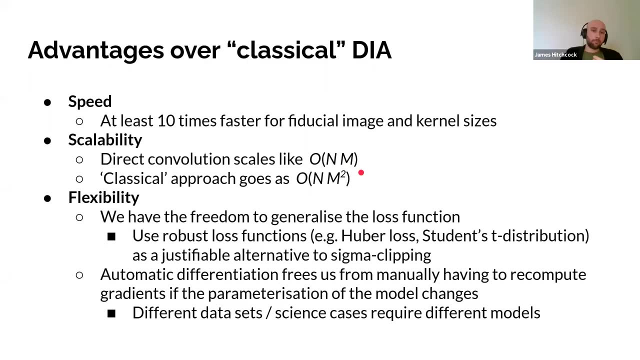 direct convolution. There can be efficient, albeit not necessarily deterministic, algorithms for doing these computations faster than this. But a third- and again I think this is another really key point here- is the flexibility of our approach. So, because we're working in an 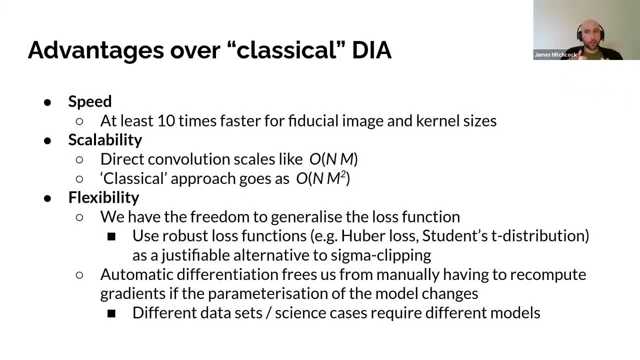 optimization framework. we have the freedom to generalize the loss function we're optimizing. So this allows us to use things other than Gaussian noise models. So the Gaussian noise model does require an optimization anyway because of that non-linearity, but we can also drop in. 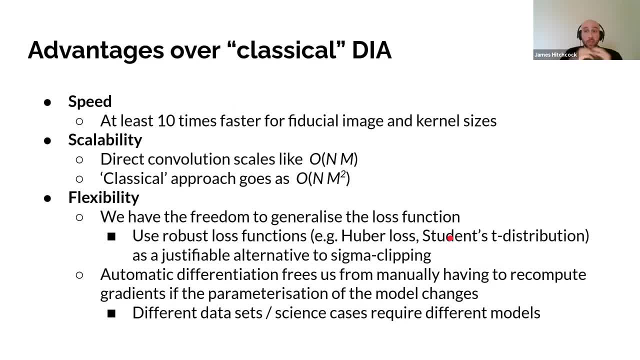 wide tail distributions if we're working with data in the presence of outliers or indeed robust loss functions that are less sensitive to outliers. So wide tail distribution like a student's t-distribution or some heuristic robust loss function like a Huber loss. Basically, the Huber loss treats inline data points. 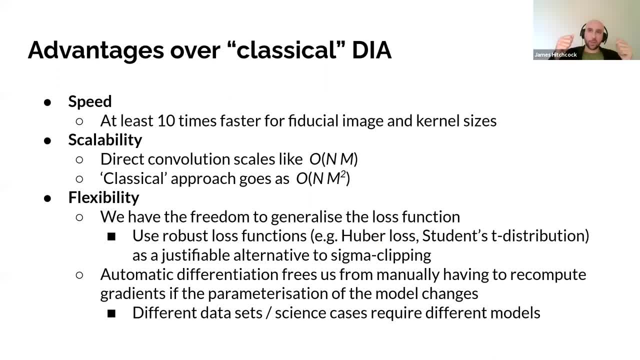 as it minimizes the square difference between inline data points in the model and it minimizes the absolute difference between outlying data points in the model, So it's just less sensitive to bad data. But these of course both provide justifiable alternatives to sigma clipping. 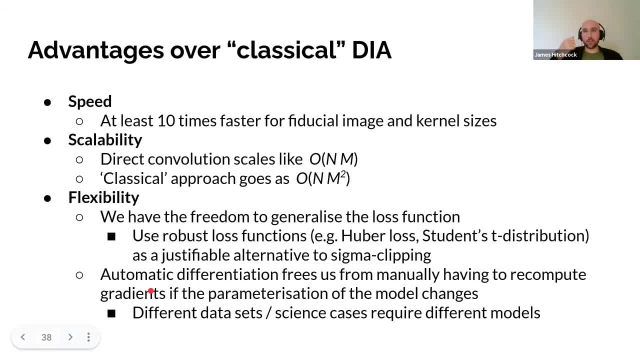 And lastly, because our approach makes use of automatic differentiation, we have a flexibility here to change up the parameterization of the model and cater it to different science cases. And again, as all gradients are done automatically, this makes experimentation and development quite streamlined, as you have the luxury to play around with. 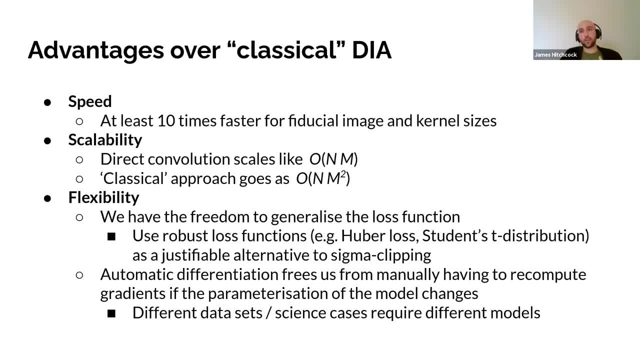 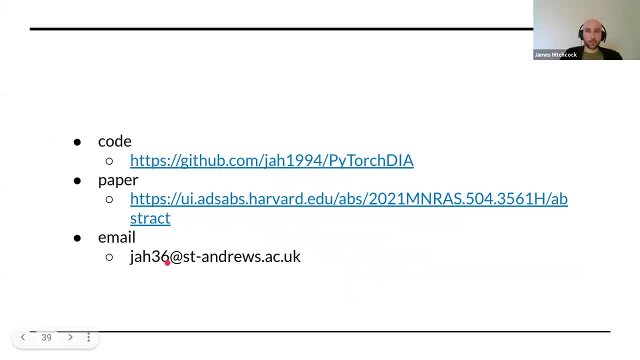 different models without having to worry about manually recomputing gradients each time you want to try fitting that to some given data set, And so that's all for me. I'll just leave you with a couple of links to the coding paper and my content details. So thanks very much for listening. I'm happy to take questions now. 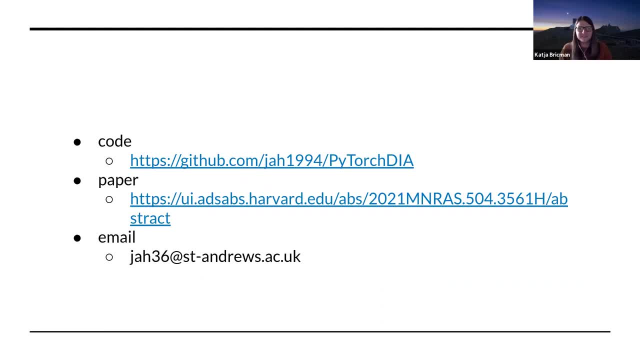 Okay, thank you, James. This was very interesting. So do we have any questions already from the audience? Yes, there is a question. Question from Yanis. Please go ahead. Hi, James. Well, thanks for the talk. So I just wanted you to comment a little bit on the kernel. 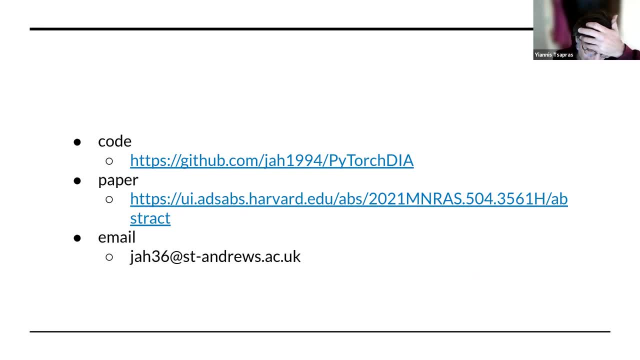 size. So what determines the kernel size that you want to use in these reductions? Because obviously if you use larger kernels then computation time increases significantly. So what determines, sort of you know, how small can you get in terms of the kernel size? 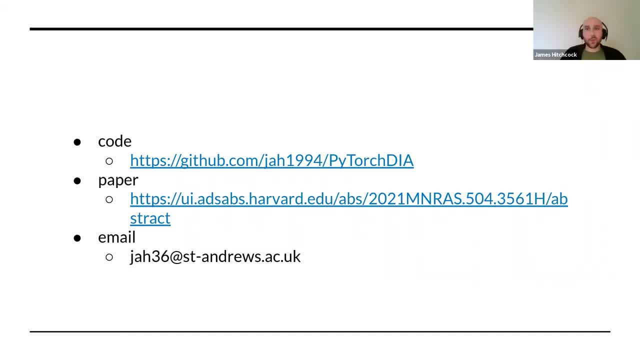 Yeah, that's a good question. So from experience I mean: so there are. this is sort of a heuristic decision that's baked into a lot of pipelines, right? So normally we say, you know, in order for a good subtraction we want a kernel that is: 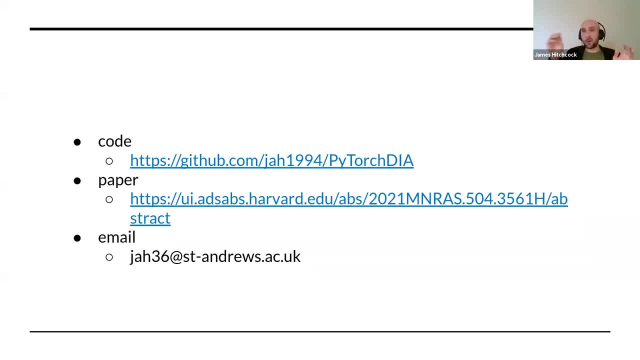 you know so many times the full width, half-maximum. So we want a kernel that is, you know, the width, half-maximum of our data image. Of course, the larger the kernel object you can specify, you know the best of the capability of the model to capture. 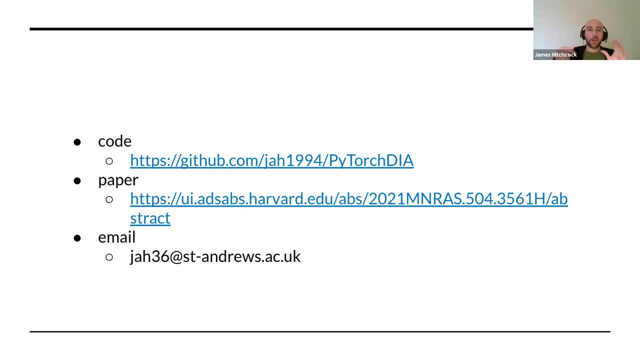 the true variation, the true difference in the point spread function. Yeah, it's. I mean, what's nice about the scaling with the direct convolution computations is that there isn't this dramatic computational overhead as you start increasing the size of the kernel. right, Because we're no longer. 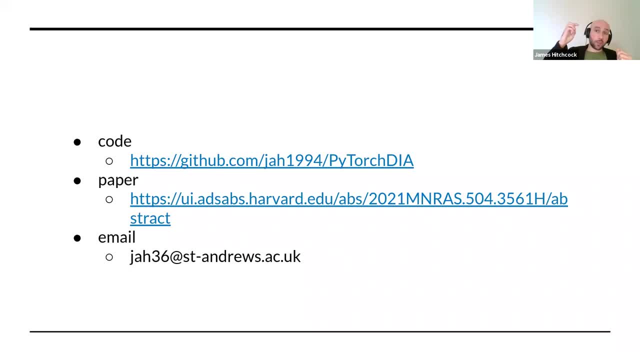 having that square difference. So this can be particularly useful if you're working with high resolution cameras that have you know very many pixels, So you can actually work with you know kernels that would just be totally impractical to use with. 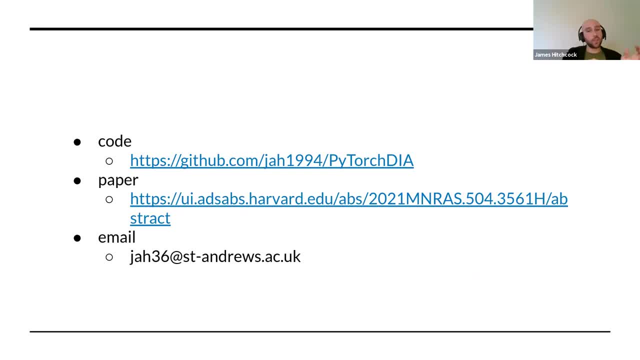 you know classical approaches, having to construct the design matrix, But yeah, the minimum kernel size. I don't know if there's like any good rule of thumb as to what determines that. I guess it just depends on your science goals and the quality of the photometry. 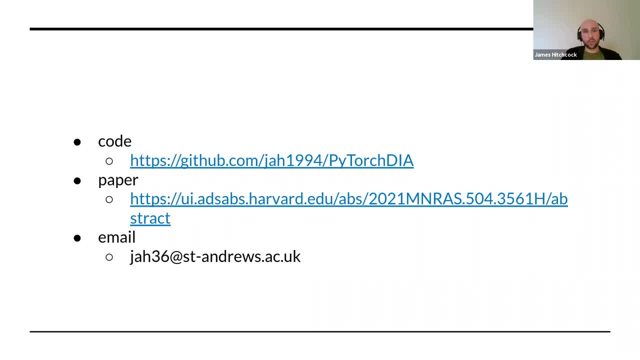 and time constraints at the end of the day, Okay, thank you. All right, there's a question from Rachel in the chat. Do you want to say it out, Rachel, or should I read it? I can pose it myself. Hopefully you can hear me. Great, So I was. 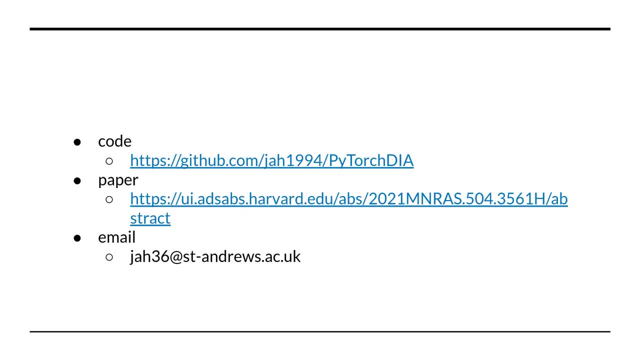 thank you for this presentation, James. It was fantastic and super interesting And I'm excited to know coming from an observer's point of view. I'm only too well aware of just how widely variable image data quality can be And I'm wondering how well the algorithm copes in. 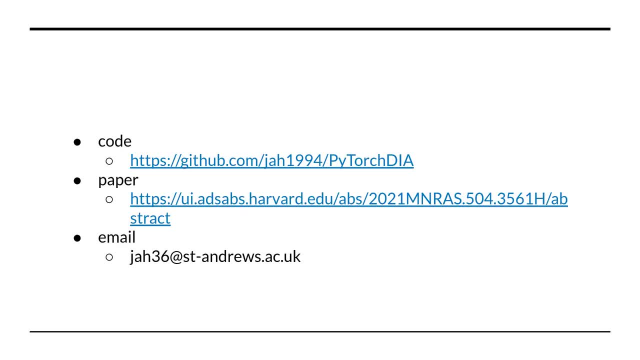 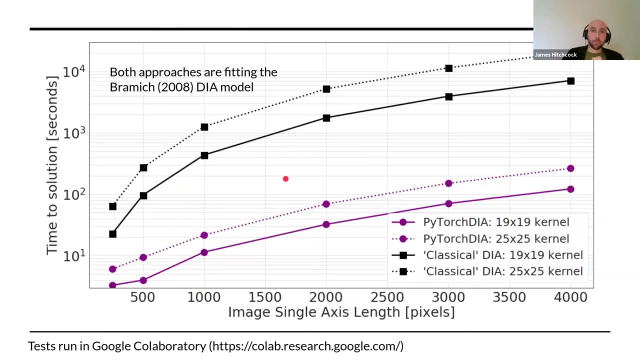 practice with things like variable sky background? What happens when it's non-uniform? Yes, so this. so I should just say all these performance test results. the model that we use is just a scalar for the sky background, But you certainly can, you know, you can, you know, you can. 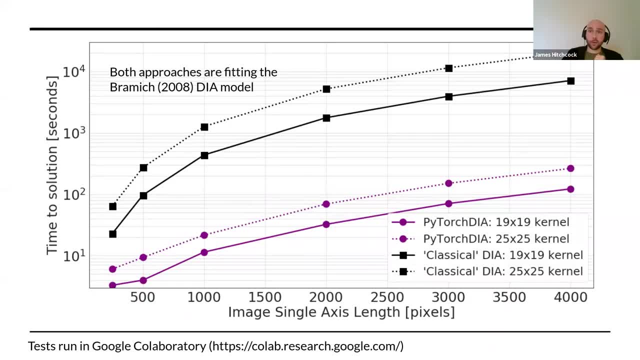 implement spatially varying sky backgrounds. We do that in PyTorch DIAs. There is an option to fit like a polynomial representation of the sky background. Of course, the optimization problem becomes somewhat trickier. And yeah, that really particularly because of your choice of initialization, because it's a priori. it's difficult to know what those 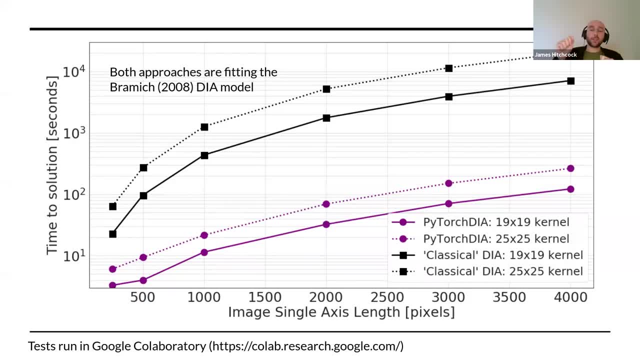 poly what values those polynomial coefficients do take. So you know some experimentation is required. but hopefully you know data sets, will you know? share some, some commonality. If you're working with you know some data set, they should be around the same sort of value. So 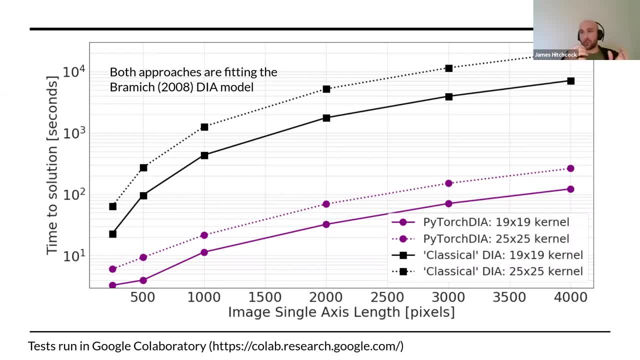 I just, I'm just talking from experience, from working with some data, So you, you do eventually get a good idea of what they, of what those should be approximated at as initially. But yeah, it does require a bit of heuristic experimentation. 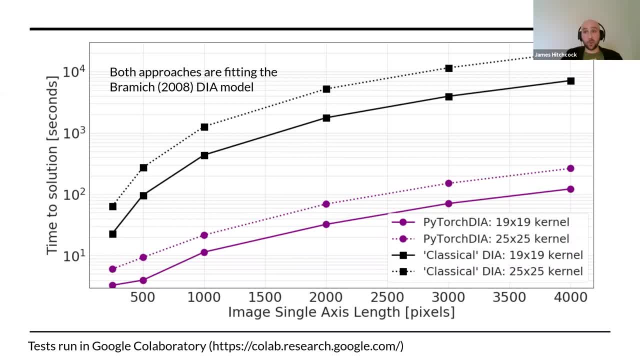 as there is an extra human overhead there if you're working with spatially varying backgrounds. Thank you. We have another question from Bruno Hi James. Excellent work, Really nice. So I wanted to know if the algorithm that you're using would support- I don't know if it supports already. 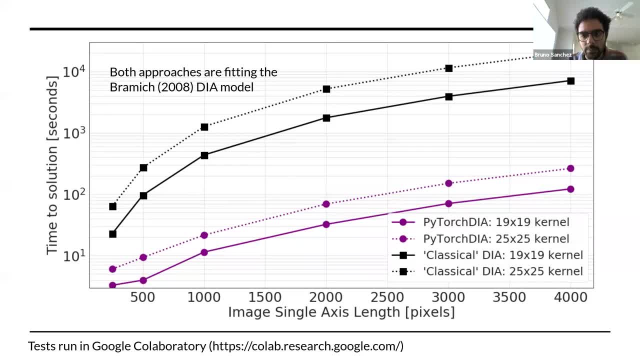 regularization on the kernel like any kind of penalty on that. Yeah, So that that's again pretty straightforward to achieve because of this- the auto automatic differentiation tools. So it's straightforward to just add whatever penalty you would like to any reasonable penalty onto whatever loss function you're optimizing. 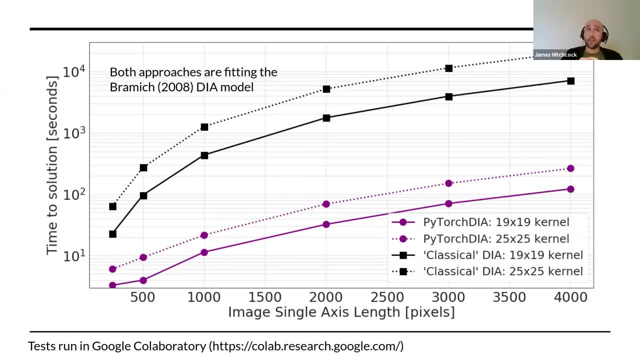 So in the in the code PyTorch DIA we introduce the Laplacian regularization onto the kernel pixels, which is basically like just the connectivity graph on the kernel. So it favors, you know, pixels to have similar values to the neighbors, So you get smooth kernels. 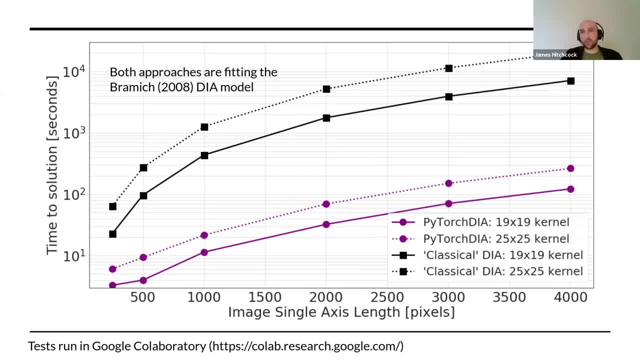 but it's. but it's straightforward to just implement. you know, straightforward L2 or L1 norms on the kernel pixels also. Thank you, Okay, Are there any questions left? Yeah, There is a question from you, Hi. So my question is: does this approach produce less artifacts than the traditional method? 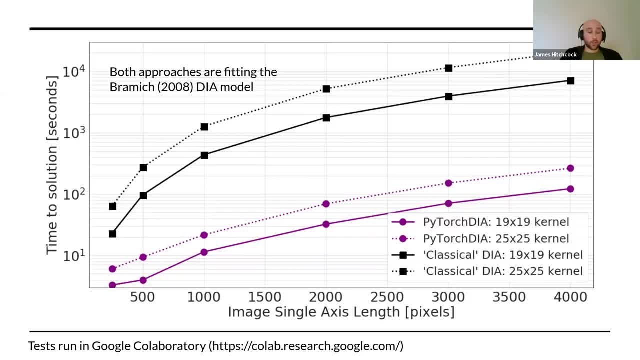 So so, yes, So one major source of artifacts- again I just talking from personal experience- is that your convolution kernel isn't large enough. And again, what's what's nice about this approach is that you, you it's it. it scales much better with larger kernels, So you can sort of get away with. 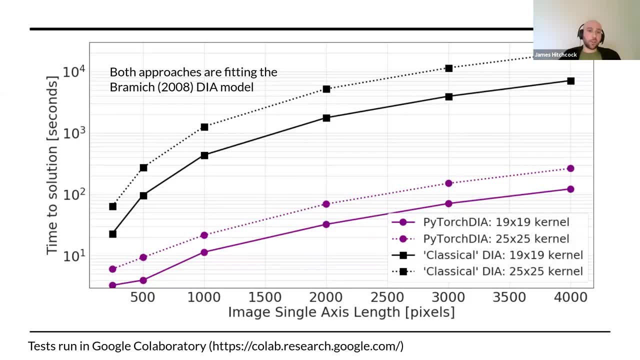 experimenting with larger models, But you know, ultimately, the image model, the model itself, that we're implementing it. they are directly, you know they are identical to, to the, the classical approaches. Yeah, I suppose the key difference, I suppose the key difference here between the models I'm implementing in this work and LSST. 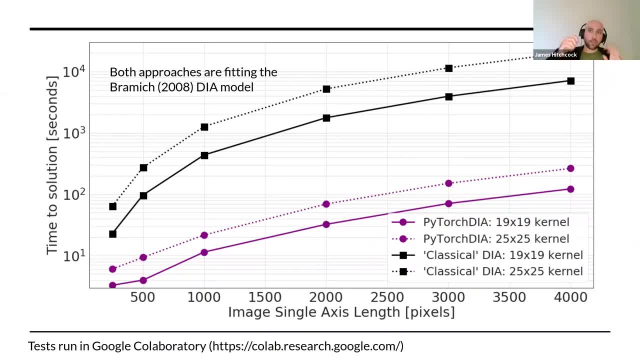 are the choice of basis functions for the kernel. So I mentioned that this is a discrete pixel array, a model for the kernel which is more flexible than the Gaussian basis functions used in LSST. So you know that's useful if you're working with somewhat irregularly shaped PSFs. So I'm not sure. 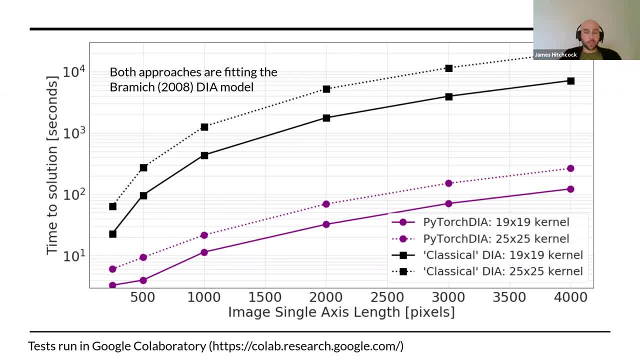 how if that's the case for LSST. But yeah, other than that, it's just the size of the object to represent the kernel. you know, because that scaling is better, that can go quite a long way to helping beat down some artifacts. 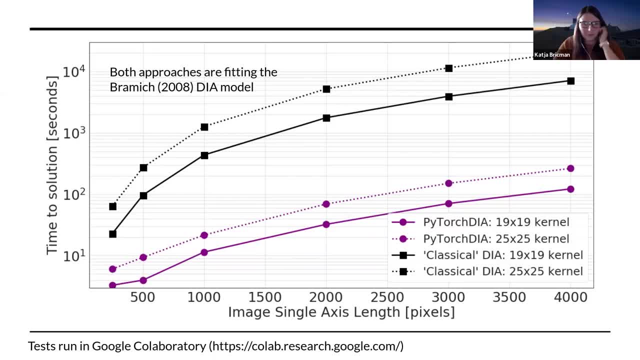 Thanks. There was another question from Yanis in chat. Do you want to say it out loud? Yeah, sure, Have you run any comparisons Of the photometric quality of the crowded-field stellar Likerts that you get from your method with those obtained from standard PSF fitting algorithms such as IRAF or you know? 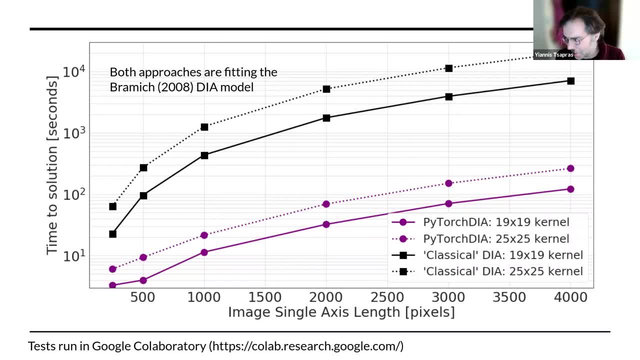 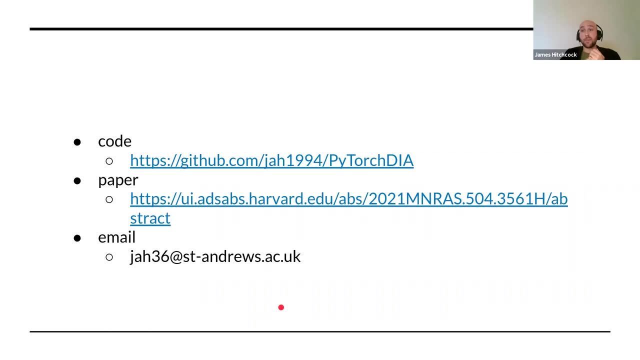 DAOFOT, Or do you not intend to do so, because DIAs generally outperforms PSF fitting in very crowded fields, Or do you plan to do something like that? So I haven't done the direct comparison against PSF fitting photometry, But I think it's a good question. I think it's a good question. I think it's. 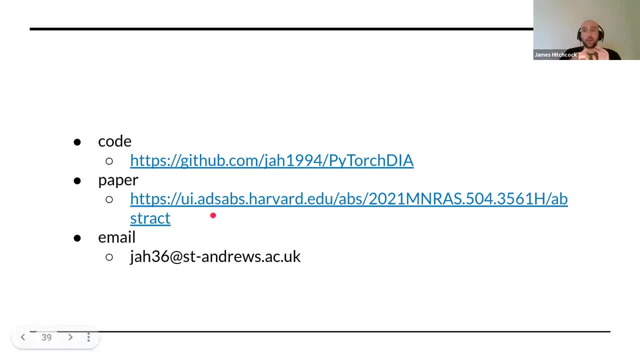 a good question, But in the paper we do do a direct comparison between its classical analog. We don't do the comparison at the level of the light curve but we do use, you know, proxy metrics for that that give an indication of quality. And you know we do show, you know. 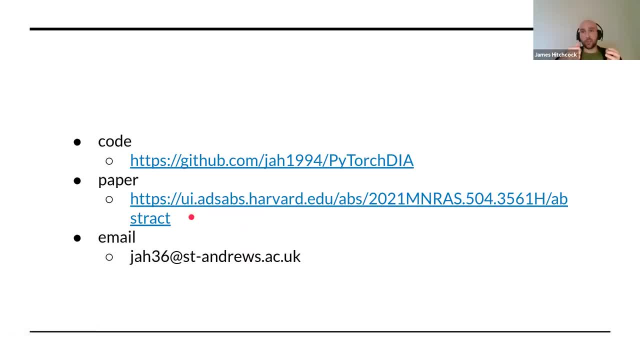 equivalent photometric performance at the level of precision that you would typically reach, you know, with conventional imaging. somewhat less precise, but at a level that doesn't really matter because we, as we're running computations on the GPU. in order for these to be fast, we need to work at single floating point.